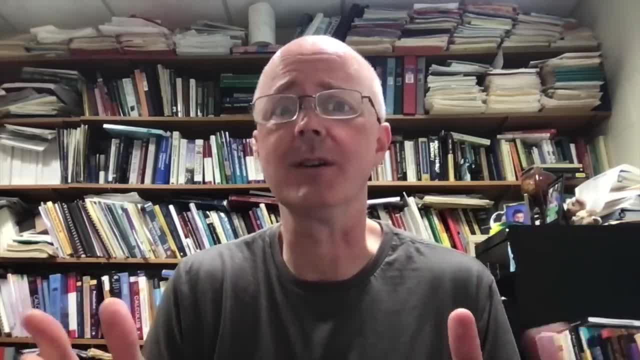 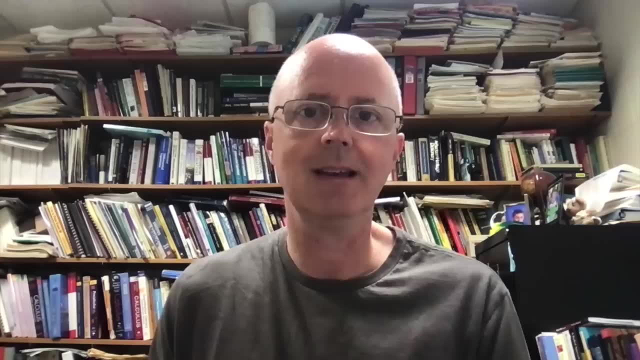 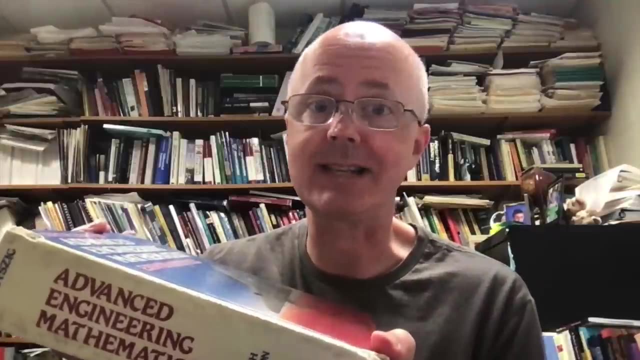 What is the hardest math class in the world? Is it calculus? Well, in spite of what my babysitter told me when I was seven years old, the answer is no. Is it advanced engineering mathematics? In spite of its thickness, the answer is no. How about the advanced math major subject called? 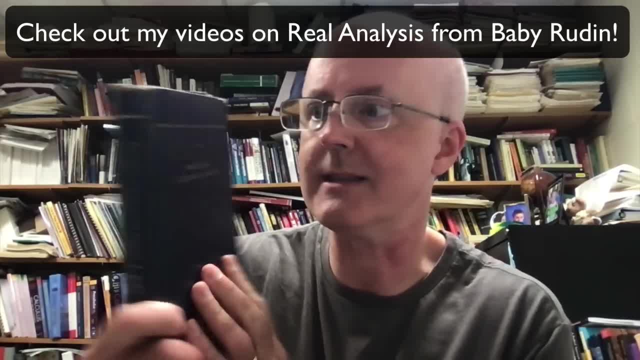 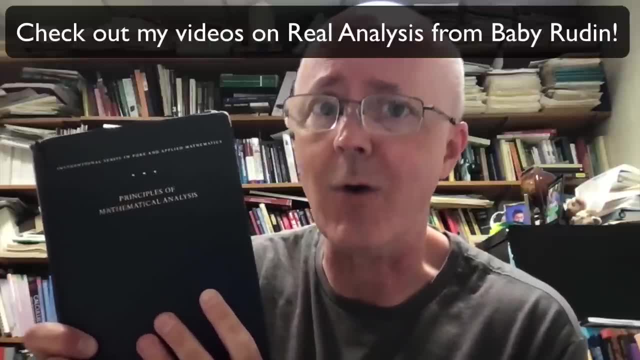 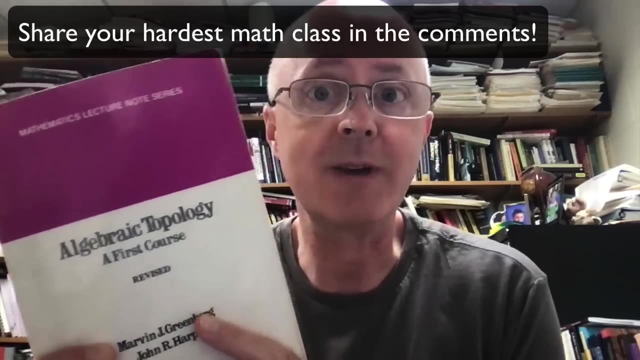 real analysis that will often come to you in thin books like this. Such pain and misery coming from such a thin book. Well, believe it or not, the answer is still no For me. my hardest math class was my third quarter of my algebraic topology class, when we got a new professor who decided 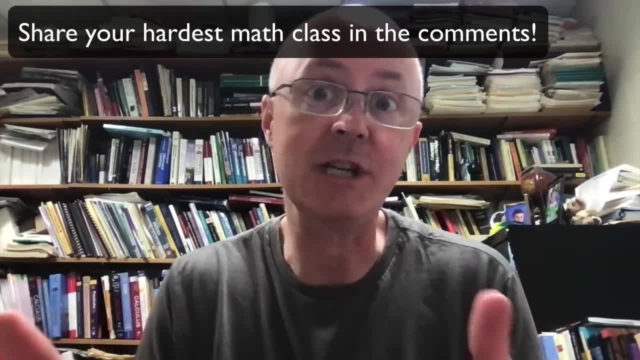 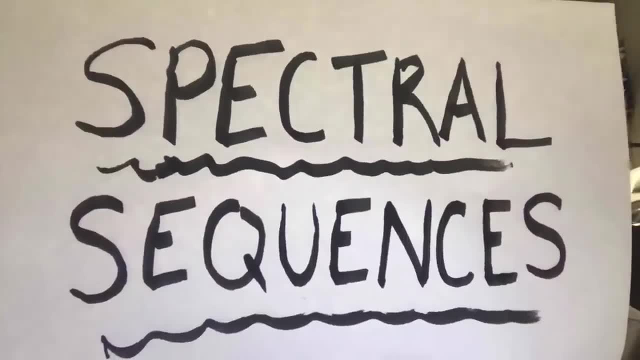 to veer off from the main content of the book on homology, cohomology and the fundamental group, and decided to devote the entire quarter to the study of- well as Darth Sidious would say- spectral sequences, Both algebraic topology and 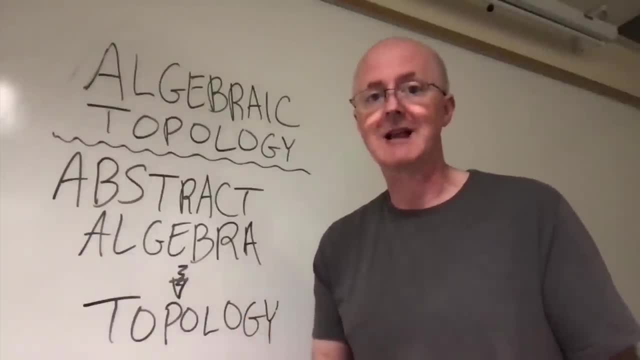 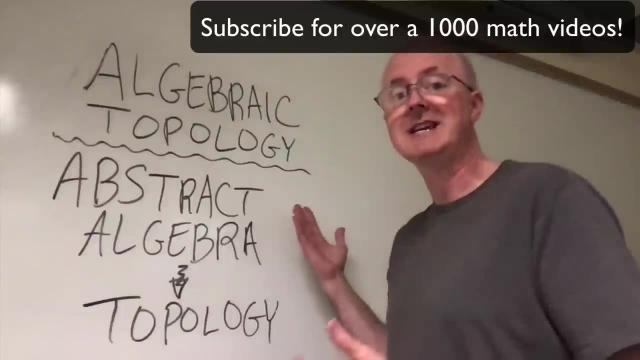 certainly. spectral sequences are examples of graduate-level classes in math. Before we get into what happened in my class on spectral sequences, we should briefly look at what algebraic topology is In a nutshell. algebraic topology takes abstract algebra groups, rings. 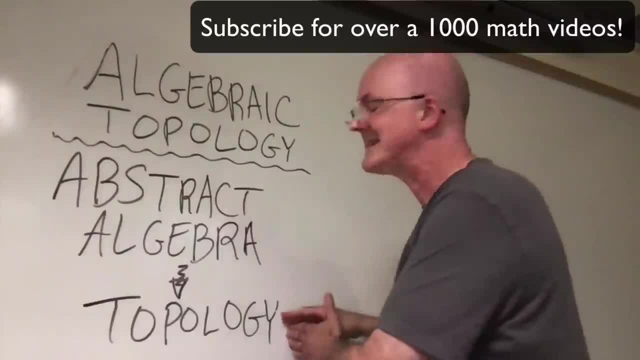 fields, certainly more advanced than what you learn in high school, and applies it to the study of topology, which, in general, is the study of abstract space, though you can apply it to, for example, surfaces like a sphere or a torus. 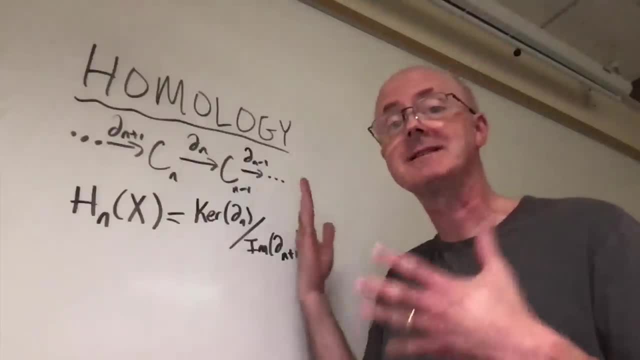 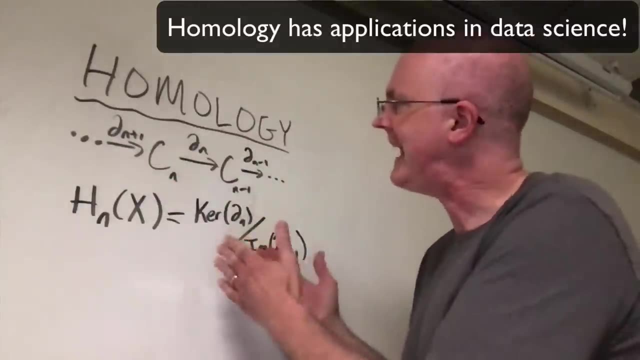 To go into a little bit more detail. homology is an example of a subject within algebraic topology where you form essentially infinite chains of groups and then take those groups and form what are called homology groups of a given space. x. This homology group tells: 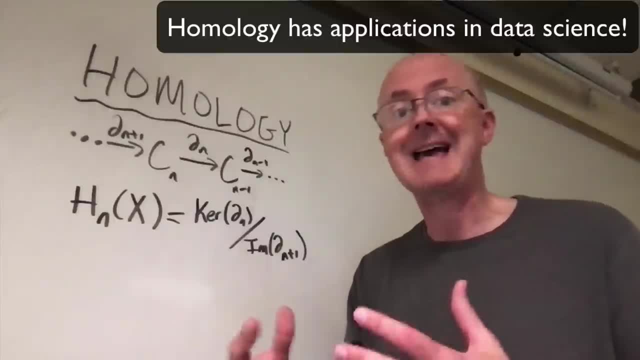 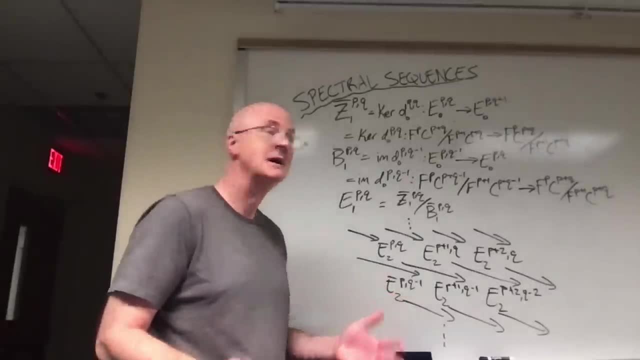 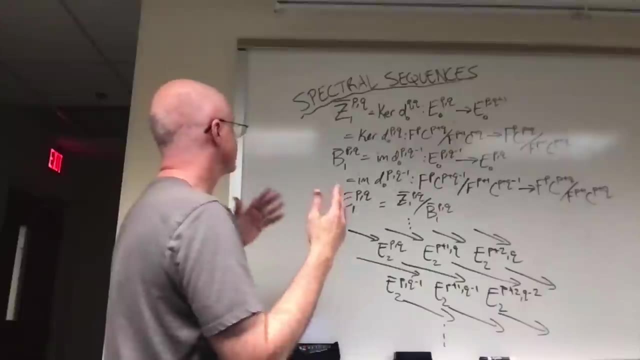 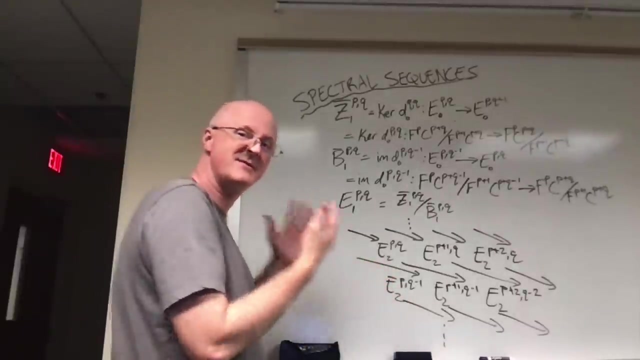 you information about the space, perhaps how many holes the space has in it of various dimensions? It turns out spectral sequences are actually ways of computing homology groups. but you can see it's much, much more complicated. Transcript 1: The letters often represent groups, The arrows represent homomorphisms. This filled the board.